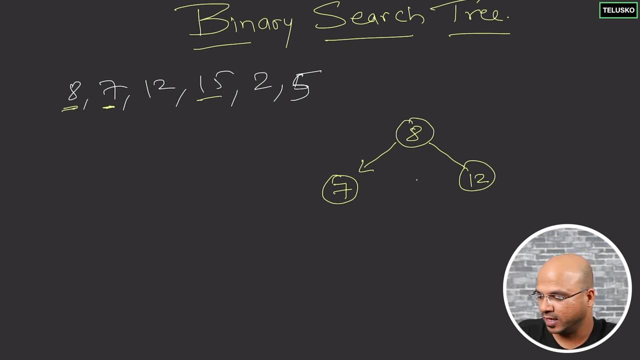 What you do is you travel Now where to travel- Left or right? Now 15 is bigger than 8, so it will go on the right hand side, But we already have 12 there. Now 12 have an option of putting 15 left or right Now. since 15 is bigger than 12, it will go on the right. 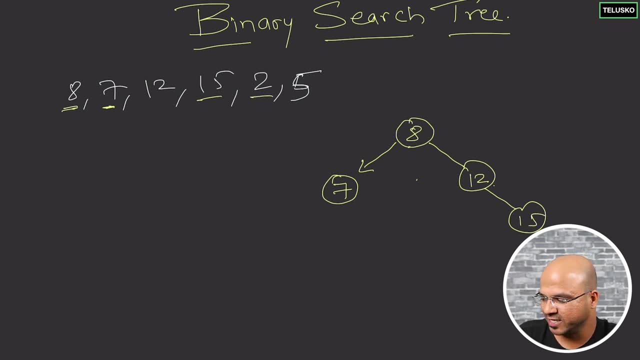 hand side. So 15 goes here. Next element is 2.. Now 2 is smaller than 8.. Again, we are starting from the root node. So starting from 8, it is smaller. Then it goes to 7. It is smaller. 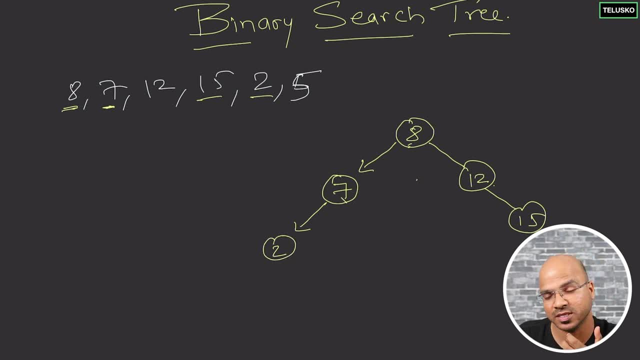 It goes on the left hand side of 7, which is 2 here, because it is less than 7. So it goes to 7.. Next we have is 5.. So we go to 8.. It is smaller than 8.. We go to 7.. It is smaller. 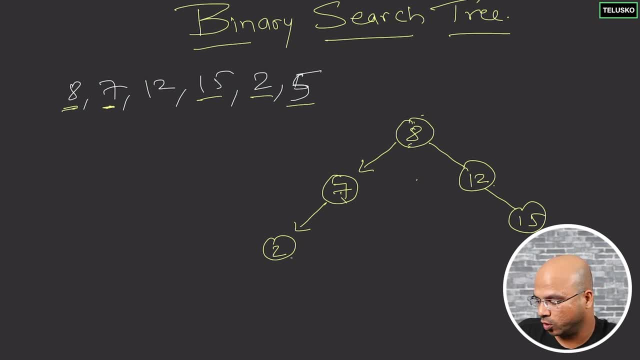 than 7.. We go to 2.. It is greater than 2.. So it goes on the right hand side of 2.. So 5 goes here. So this is how the binary search tree works. Now, once we got the basic understanding, 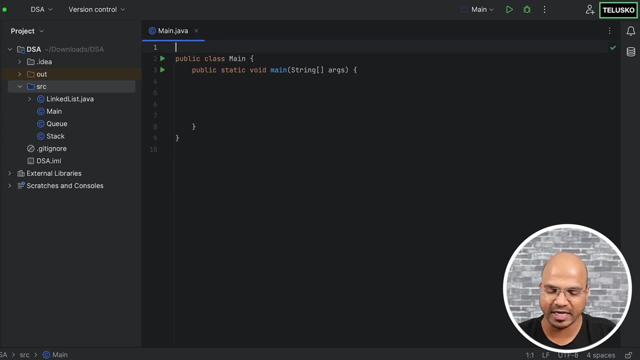 let's start the implementation. If I want to code that, first of all we need, for sure we need- a class called node, right? In fact, I will not be writing this here, Let me just remove it. What I want is I want from my main method. basically, I want to create a binary. 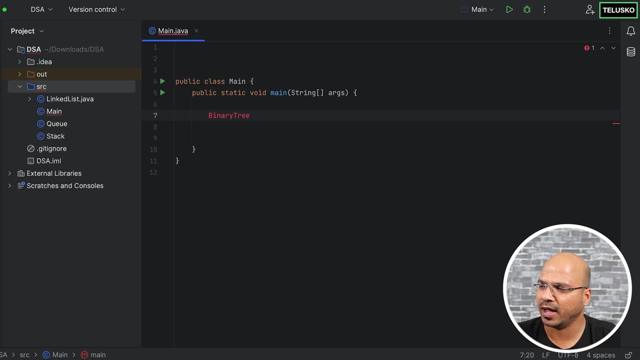 tree. We have some inbuilt classes, but we are not going to use it. So let's say binary tree and we will call this as a tree equal to new binary tree. So we want to build a binary tree. You can see, we have some inbuilt methods. We don't want to use them, So let's use a. 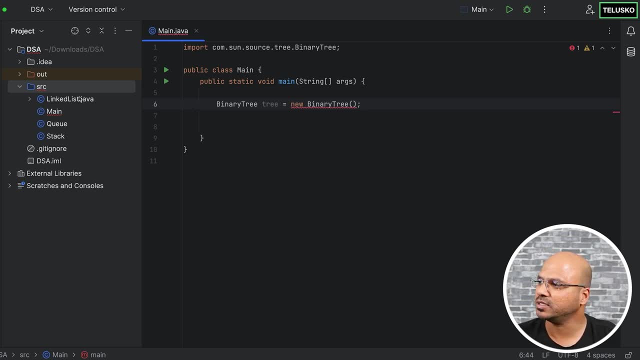 binary tree. We don't have this class yet. So what I will do is I will just go back here and you can see it is importing this package. We don't want any inbuilt things. So if I go back here and if I say, hey, give me solutions, More actions, I want to create this class. 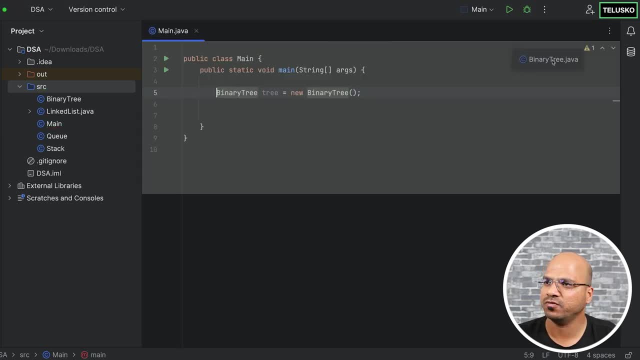 binary tree in the same package And you can see we got it. I will just move this on this side. I don't want to see the project structure. So you can see, on the left hand side we have a main On the right hand. 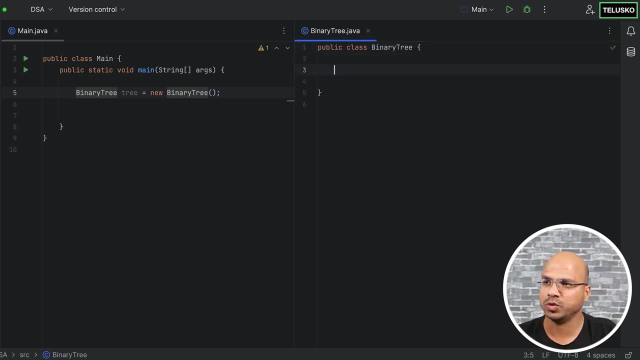 side we have a binary tree. So basically in this binary tree I want to do all those stuff. Now when I say I want to do stuff, basically we have to say tree dot, I want to insert value in this tree, So I can say insert and I can pass a value, let's say 10.. I don't know. 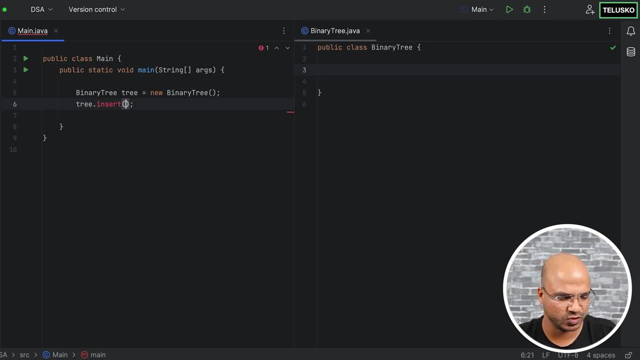 what values I am passing here, Or maybe I can. I can for the same value which we have in our node. So we have 8,, 7,, 12,, 15,, 2 and 5.. Let's add that. Okay, but then unfortunately, 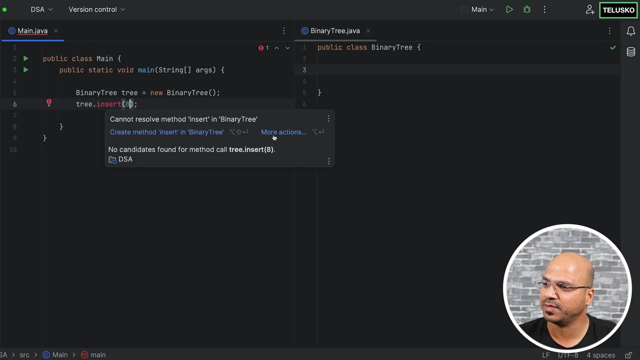 we don't have this insert, Okay. so what we need to do is we need to create this method called insert inside this binary tree And you can see we got insert method Okay. but when you say insert, that means we have to make sure that you're inserting a node Of. 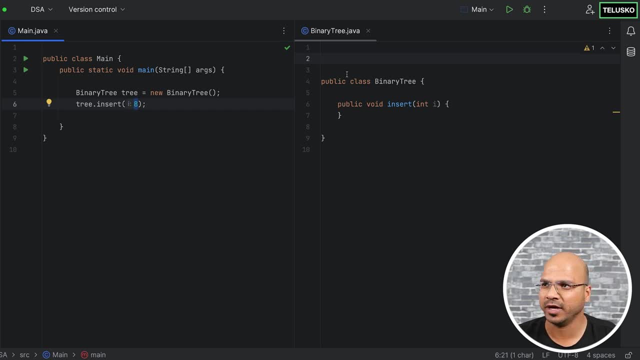 course you are passing data here, but it should be added to a node right And we don't have a node implementation yet. So I can create a node implementation by saying class node Now what every node will have. Now, if you go back to linked list, a node will have two. 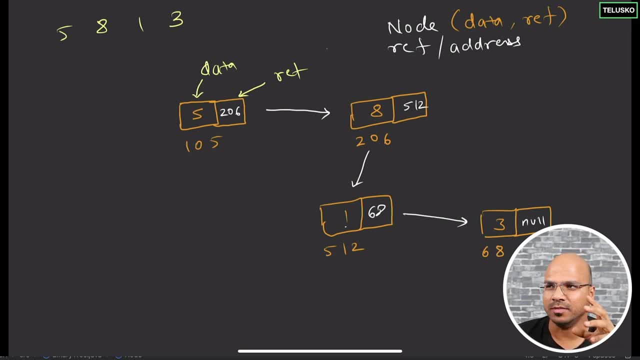 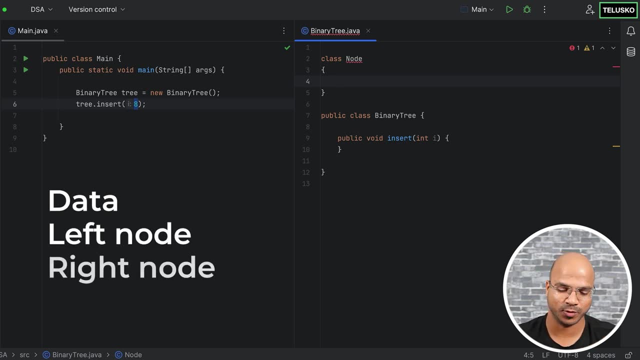 things: The data and the next value, Which is a tree node. It will have three things: Data, the left node and the right node. So I can say int data, Then we have to say node, Because when you say right node, 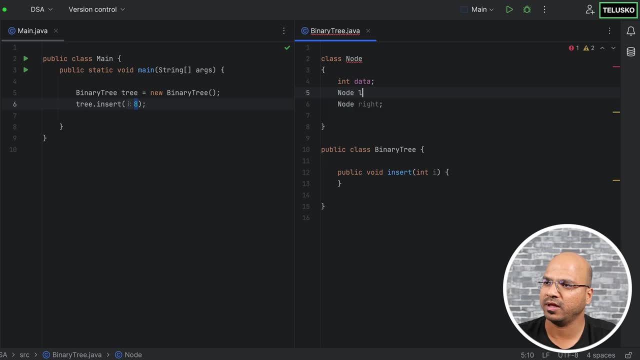 left node. they are itself nodes, right. Let's first write left and then right, So yeah, So we got data, We got left node and we can, we got right node. I think the only problem is in some of the class. I think in linked list we already have a node here. That's the 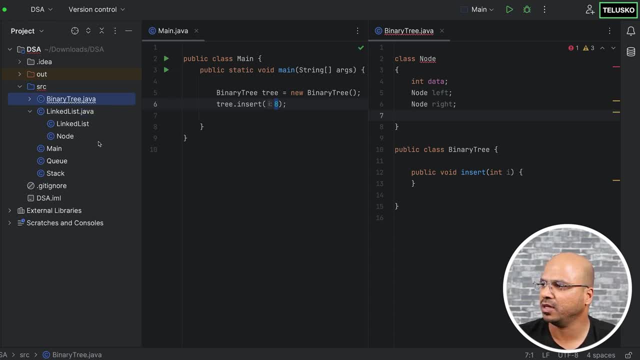 problem. So what I will do is let me just move binary tree and this main to some other package. I will just move binary to the other package, Let's say package comtelescopetree. So sometimes you have to solve the problems in a go. You need to import the package from. 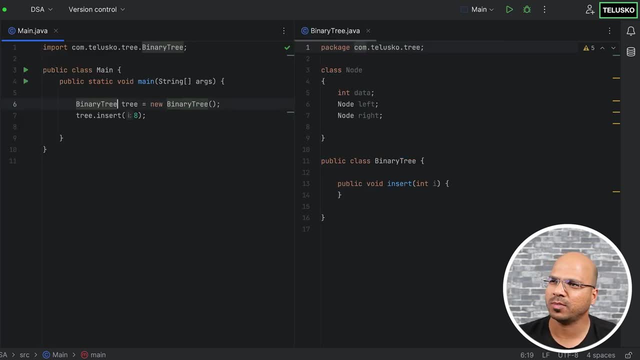 here now Importing done. Okay. So the problem was I was having two classes with the same name in the same package. I just moved it to a different package, Okay. So now you don't have to do that. if you're just writing the binary code, You can just skip this line. 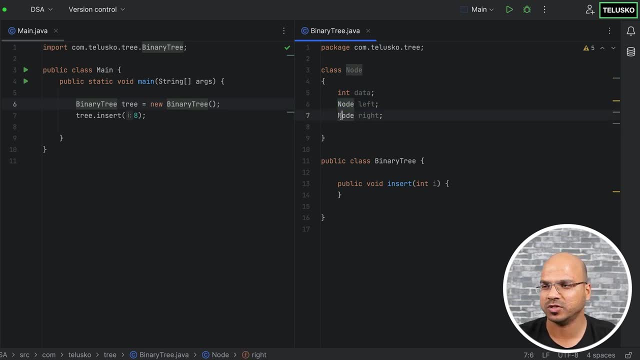 Anyway. So we got a node and then we are referring to left node and right node, So that's node done. But also, what I want to do is Maybe when I create a node, I want to have a constructor here which will take the data. 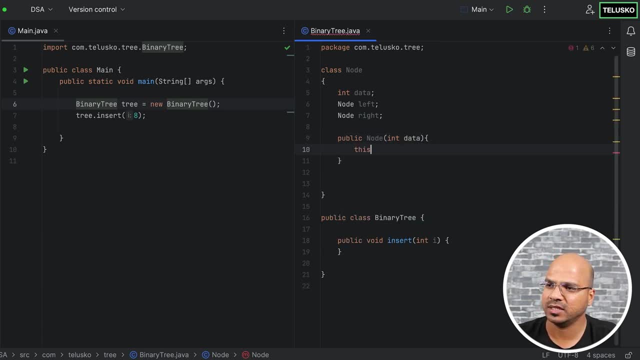 for me and I will assign that data. So I can say this: dot data to data and that's it. So we are basically done with the node concept. But how will you implement this tree? So, every time you want to insert the data in a tree, how will you do it? So if you say this is: 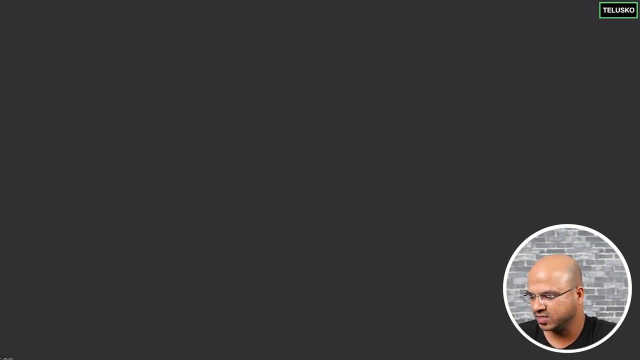 a tree? of course we don't. Let's say we don't have a tree here and let's go with the same value. I don't know what values we have, I can just use this Call Copy. Okay, So we got this value. So if I want to draw a tree, So let's say someone is giving 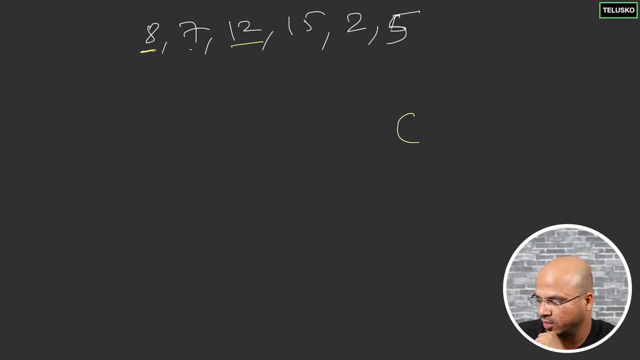 you the value eight initially. So what you do is you create a root node. Now we know that we don't have a node in the tree, So basically, the tree is empty. In that case, you will make this as a root node. Okay, So how do we do that? So when you say insert, 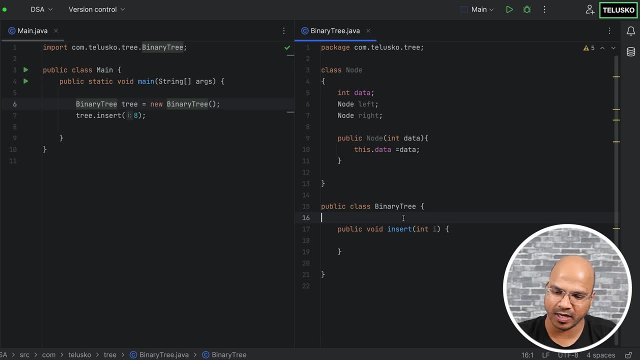 basically we have to create a root node. That means every tree need to know about only one thing, which is a root node. Right, As I mentioned before, for a tree, the most important thing is root and then tree don't have to worry about other nodes, The root node will take. 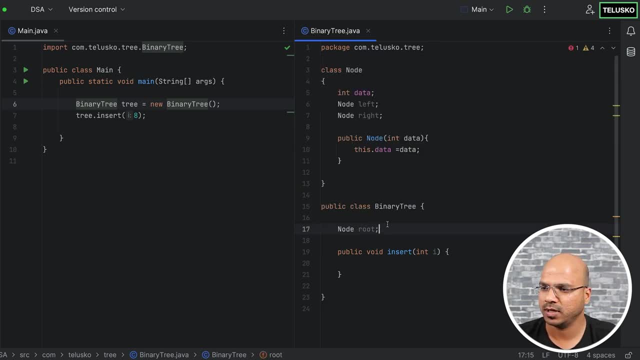 care of the next two nodes. So what I can do is I can say node root and then every time I create insert and then imagine that this is the first time. So what you will do is you will create your root node here. So you can simply say root is equal to new node. 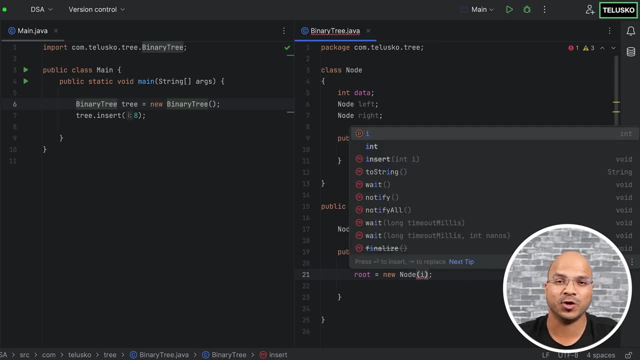 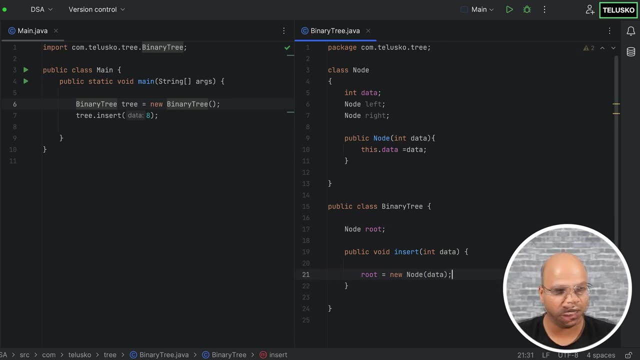 That's how you get a node: Just get the object and pass the data, and that's it. You've got your root node. In fact, you know, instead of using this variable as I, it should be data. it will make much more sense. So now, if you can see our code, this is the thing we have. 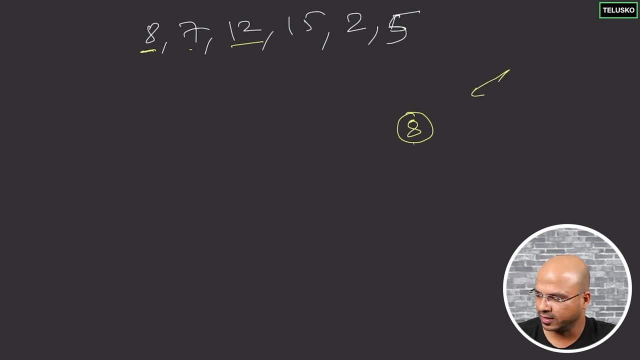 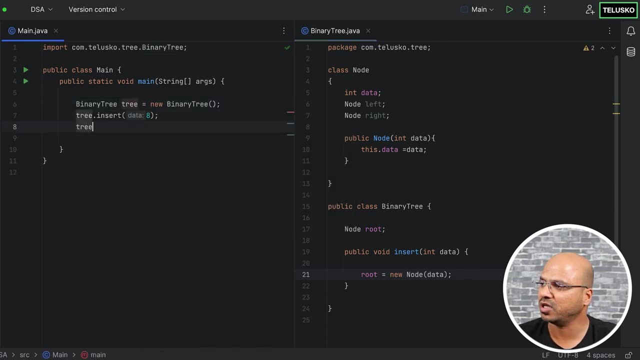 done So we created a root node called eight, and that's your root node, Which looks good. But then what about if I insert one more data here? So if I say tree insert, I want to insert the next record. What's the next record? It is seven. So when I insert, 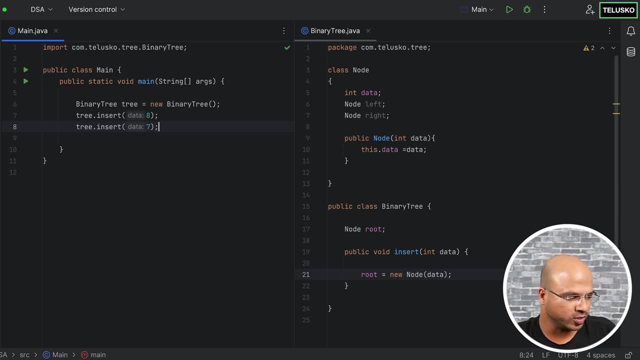 seven. where the seven should go Now don't you think the seven should go on this side- is because we are implementing binary search tree. Seven is less than eight, so it should be on the left hand side. So when I say seven, it should create a new node, and we are doing. 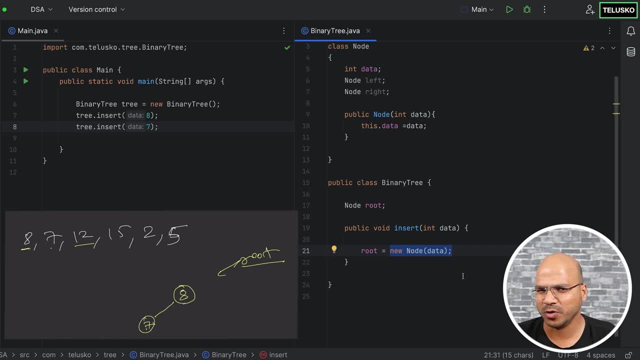 it. You can see, every time you say insert, it creates a new node. But don't you think this time is not a root node, It's a left node of the root node. How will you do that, and how do we even know that this is not a root node? So in that case, we need to do is: 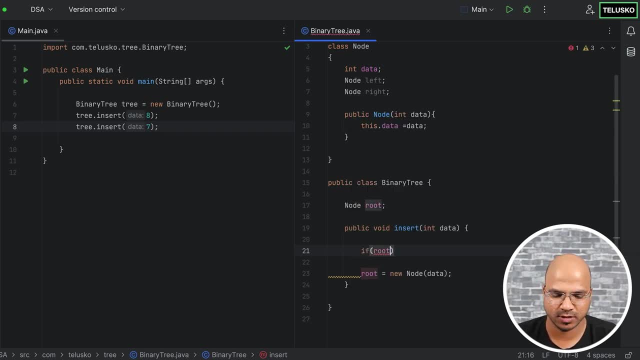 we need to check. if the root is null, Then you create a new node. I mean, then you create a root node. otherwise you don't create root node every time, So root node will be created only once. if the root is null. What else? if it is not null, then we can check for something. 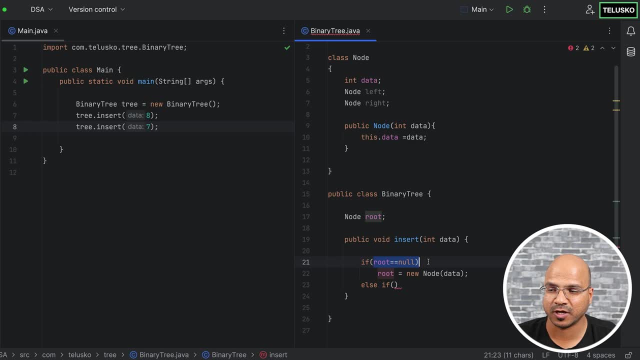 else. Now see if we talk about eight. Yes, This satisfies is because is null till this point, when you before executing 8, but when you insert 7, we already have a root node. right, then we have to go for. if else. now the question is: now we know that this is not a root. 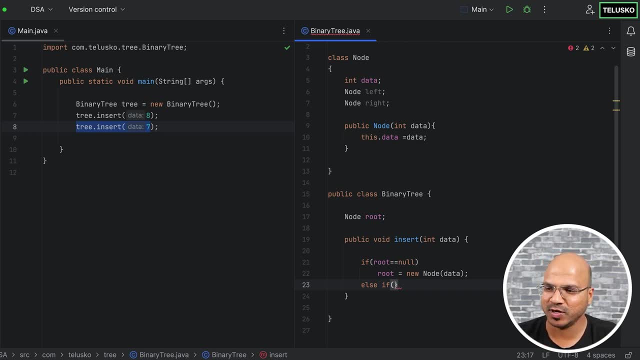 node, we have to either go for left or right. so what you do is you basically check for data. if the data is less than root dot data, then you go on the left hand side. so when you say you go for left hand side, what you simply do is you say root dot, left dot data is equal to data. that's what you. 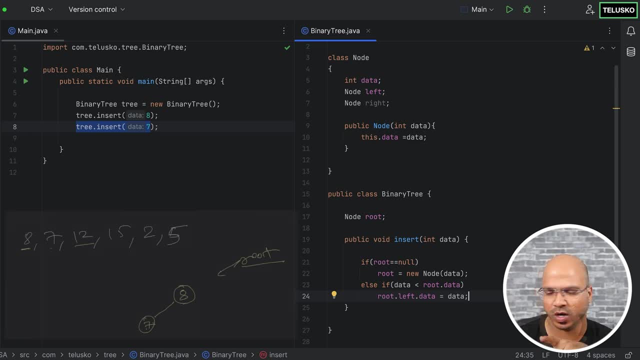 do. but then we have one little problem here, because this will work for this data, okay, so we will get new, new thing, but we are not even creating a new node, okay. so that problem is: we need to modify this to something else. why something else? let's say we have adding one more, which is 12, goes. 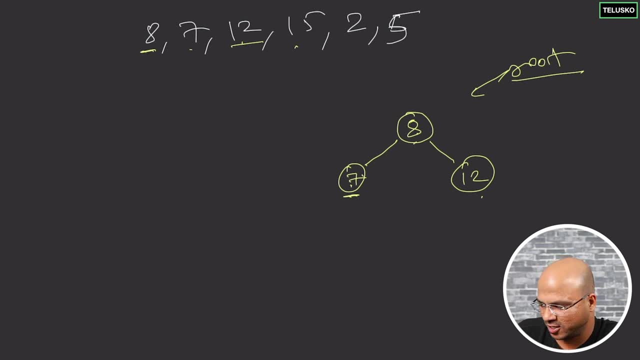 here and then you add 15. now, by our logic, if the value is greater than root node, just add it to the right hand side. but 12 is already there, right? then we have to move to 12 and it becomes a right hand side of 12. that. 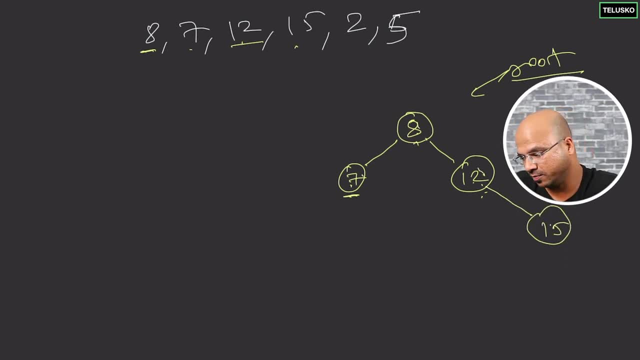 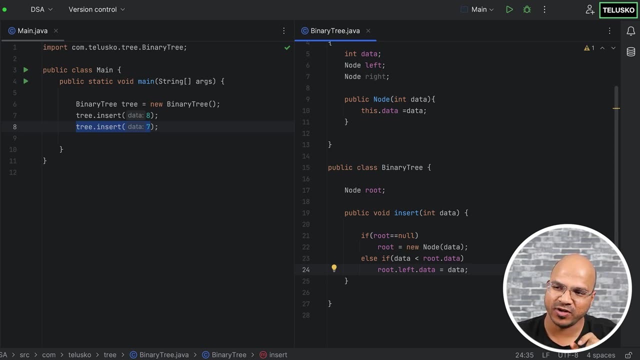 means we have to jump from root to the next element and then the next element. oh, that's a recursive process now. so that means we have to add a recursion here. that's one thing. second problem is: every time you insert data we need to get a hold on root. you know, writing the logic here is not. 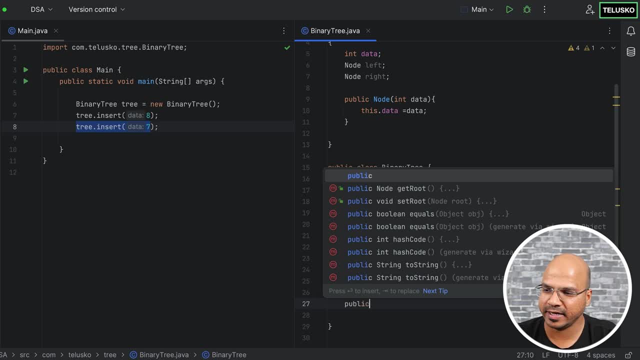 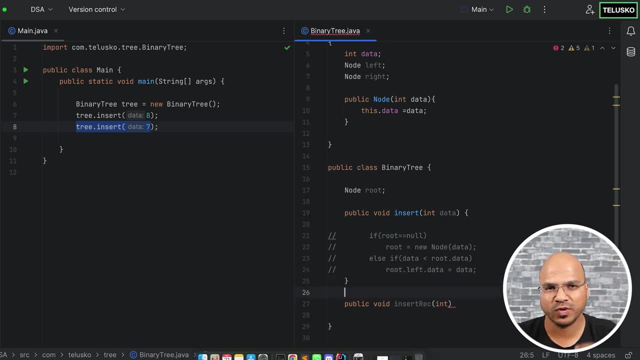 efficient way. what we should be doing is create another method which is called, let's say, insert rec, and we'll say: this will take two things. because when you want to do recursion, we have to get a hold on root element or root node. so that means we cannot do that in this insert, because the moment you use a recursion 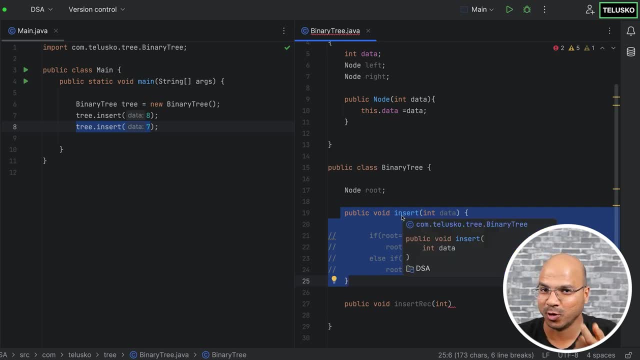 every time you call the method, we need to get the hold on the node where you're calling this. so this will not work. but that doesn't mean we have to remove this. i will tell you in some time why. so basically, we have to say node root, comma data and here, okay, this should return a node. 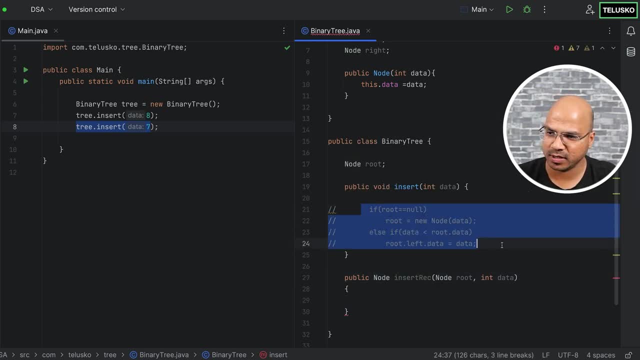 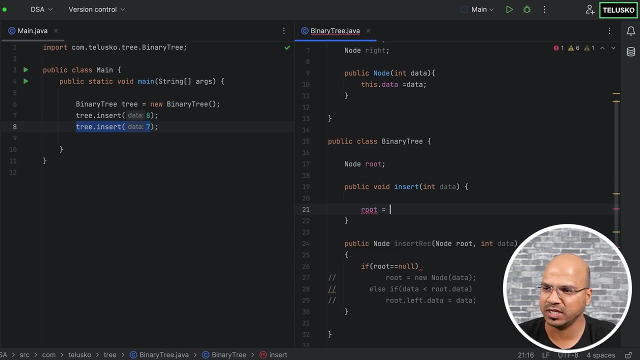 because we are going for recursion, so it should return something. and now here, instead of doing all this logic- this logic should be a part of this, not this- so here we are going to do a recursion- we can simply say: root is equal to insert record. so every time you call insert, it will call insert. 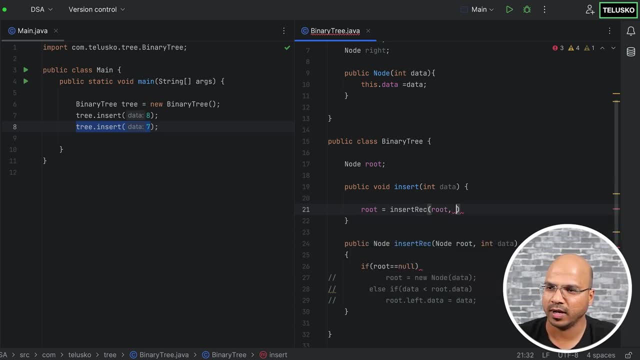 rec in which you are passing the root node and the data. so when you say recursion, it will go into recursion. we will be using recursion on insert rec, not on insert. so we have to change some logic here. so this is correct when you say root. i'm only concerned about this part. so how do we implement? 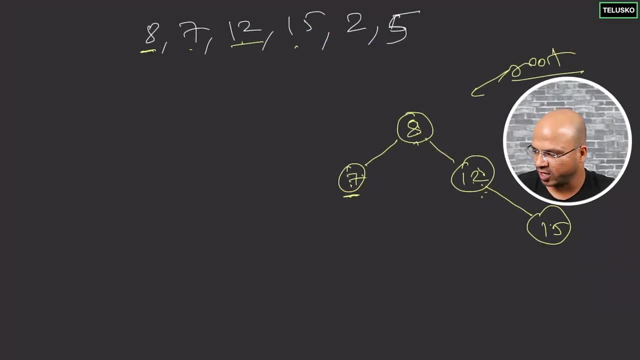 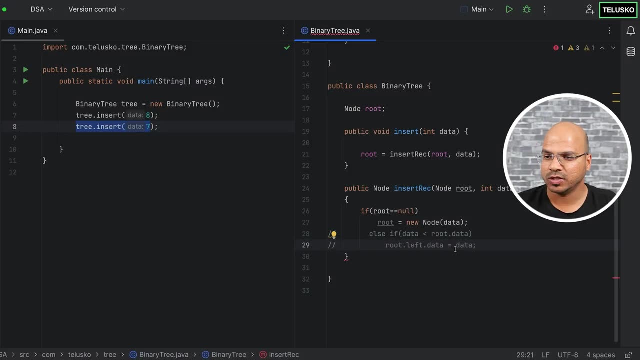 this one. so when i say i want to add element on the left hand side, so if you have, let's say two, now we know that two should go here. but let's say two should go here, so let's say two should go here, then we have to jump from eight to seven, seven to two. that's a recursive, recursive process, right? so 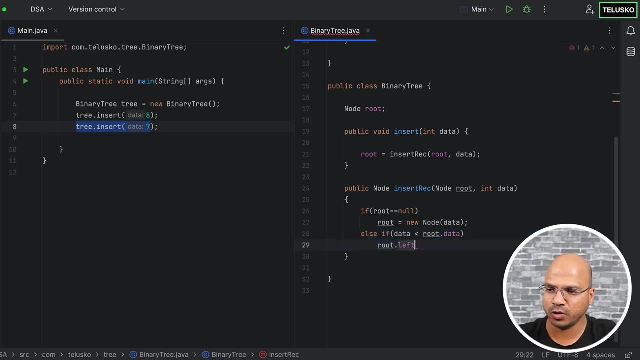 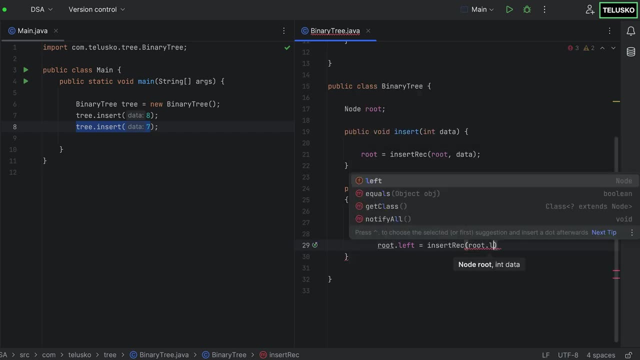 what you will do is- let me uncomment this now- this is not how you do it. so, basically, you say root dot left and then you call the function once again by passing the root dot left, because now we need to follow the tree right, as i mentioned before when you talk about the subtrees, if it 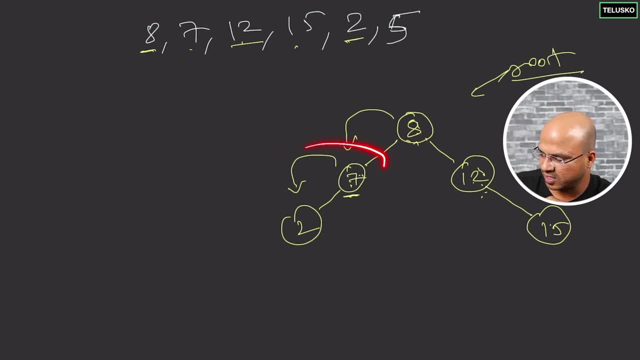 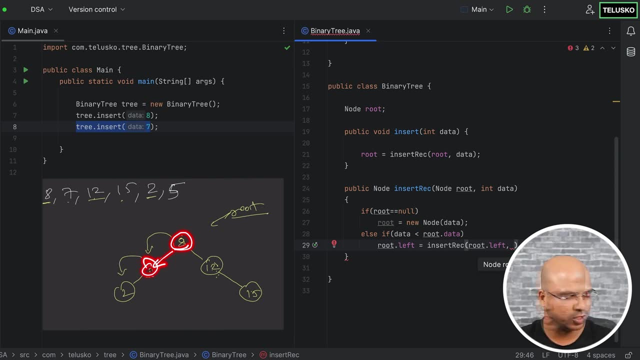 is not eight left, then we have to consider this subtree. now this seven becomes your root. so how will you send this as a root? so you have to say root dot left. now this becomes a new root. so when you call this function, which is insert rec, here this: 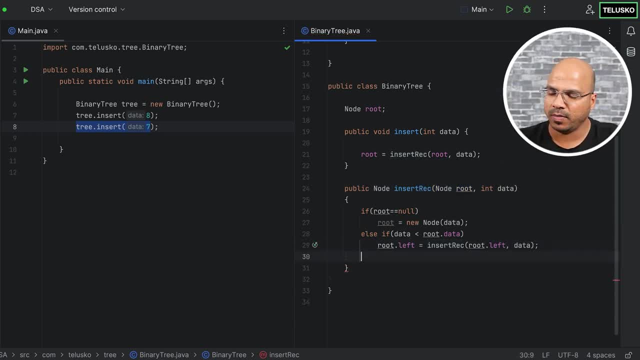 becomes your new root, and then you have to pass data as well. so you're passing data, but what if this is not smaller? then you have to go on the right hand side. so i have to say root dot data. if data is greater than root dot data, then you do the same thing, but for the right hand side. so 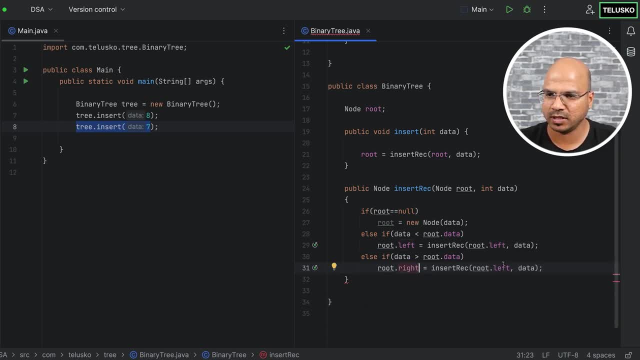 i will say: paste here. so this should be right, and this should be right. and then at the end you know your root node, so just return: root dot left. and then you have to go on the right hand side and say: root dot, dot, root dot, that's it. so this is the recursion call which we are getting here, so that's. 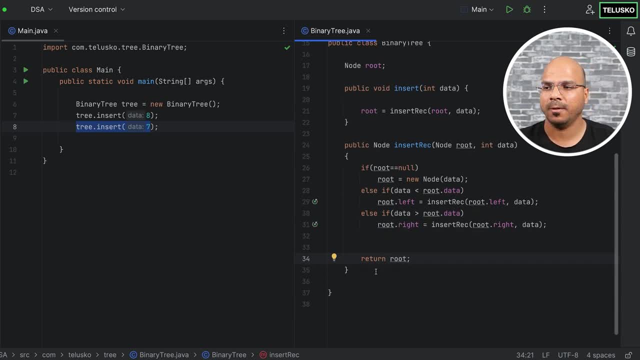 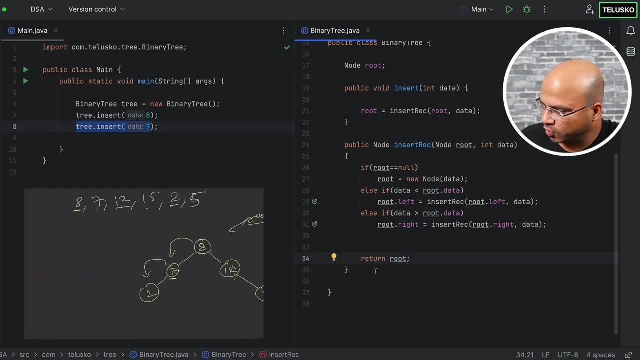 how, basically, you create a tree. now, this is tree is created, but how will we know that this tree is created? we want to print also right, and the way you can print it is like this: so if you want to print this tree, so let's say we have this tree here and this tree is created by the way we have. 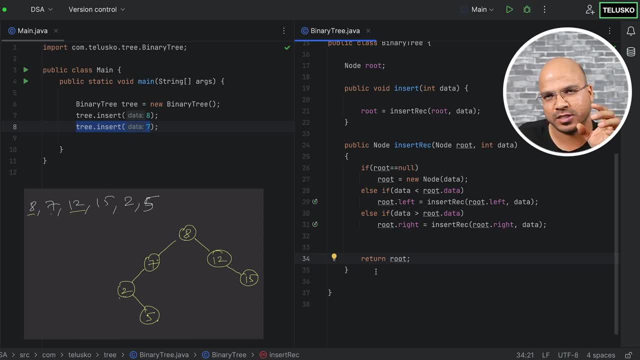 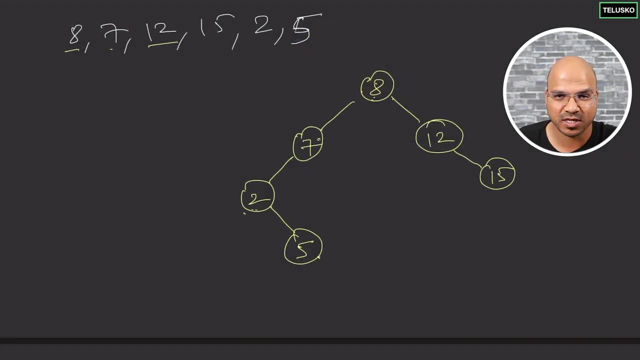 defined this example here. how will you print this now? to print, we basically have to traverse or we have to travel to different elements here. the way you do that is, we have to different travel cell for tree. so when you talk about tree travel cell, we have to follow certain 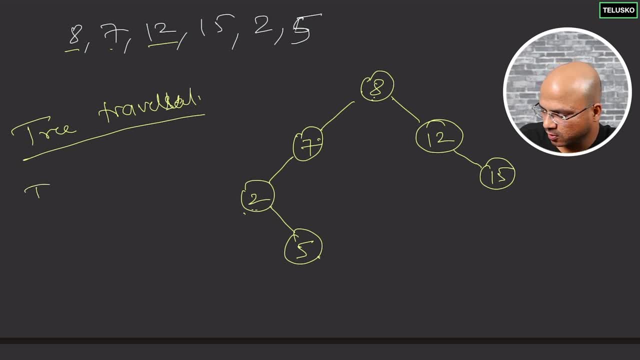 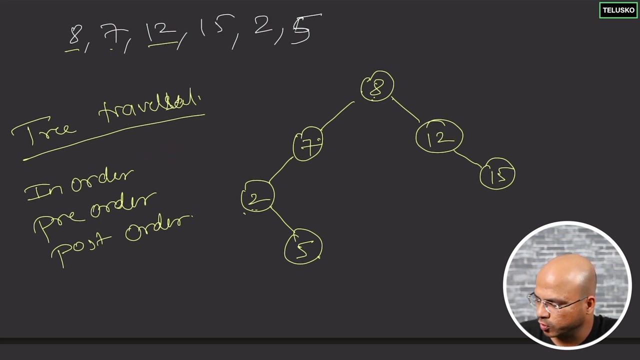 things first. there are three, three options here. we have in order traversal, we have pre-order traversal and we have post order. the difference between these three is the way you print your root node. okay, so when you talk about in order, basically what you do is you first go to the left. 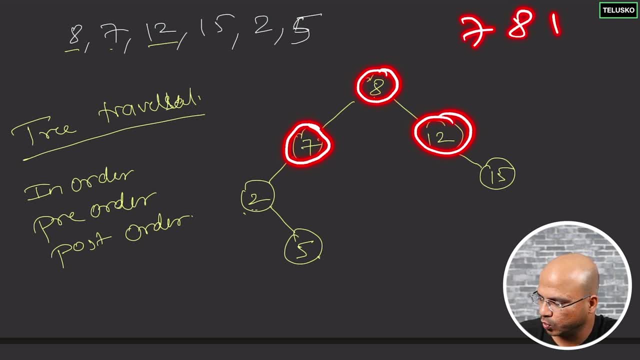 then you go to the root, then you go to right, so which is seven, eight, twelve. when you talk about pre-order, here you first go to root, which is eight, so it will print eight, then seven, which is left, and then twelve, which is right. when you talk about post, it means first it will go for left, then right. 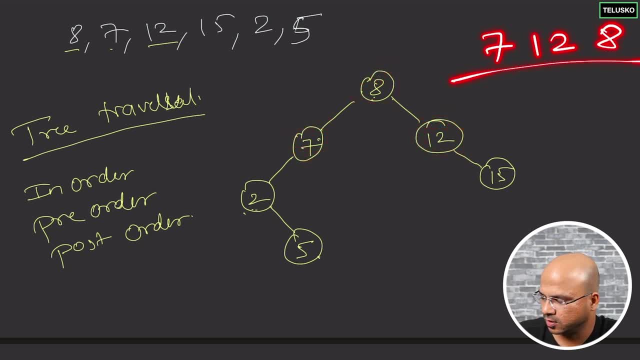 then root, which is seven, twelve and eight. okay, that's your post-order traversal. here we are going to go for in order. so in order simply means first you print the left one, then you print the, also exactly printing, but you go to the left one, then you go to the root node and then you go for the. 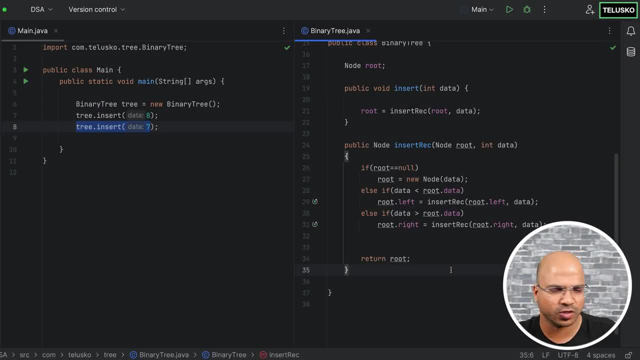 right one. so if that's your in order, now the way you can do that. of course, this is also recursive, right? uh? so in order to do that, what i will do is i will create a function called public void in order. then you can work here. but then, since we know that in order is actually or traversal, 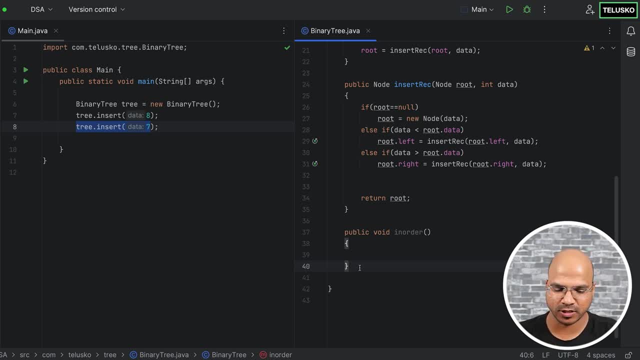 is basically a recursive operation where you go to each subtree and print it or do some operations for the recursion. i will create another method which is public. void is because i don't want to return anything. so i will say: in order, rick, so here, we just want to print it. now, when you say 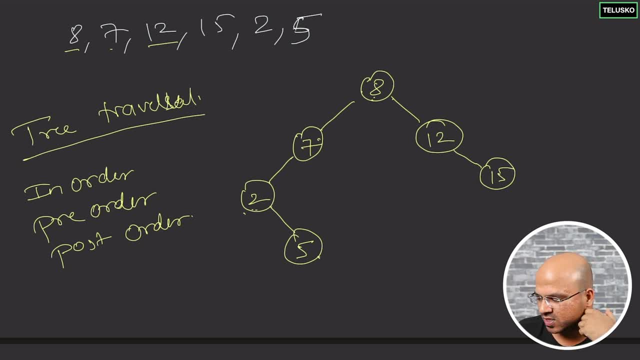 print it, how exactly we are going to print, how we are going to travel this. of course, the output will not be similar to the value we have inserted. it will have a different order. so what it will do is, first it will go for it will print the left, one right. so when you start from here, it goes to: 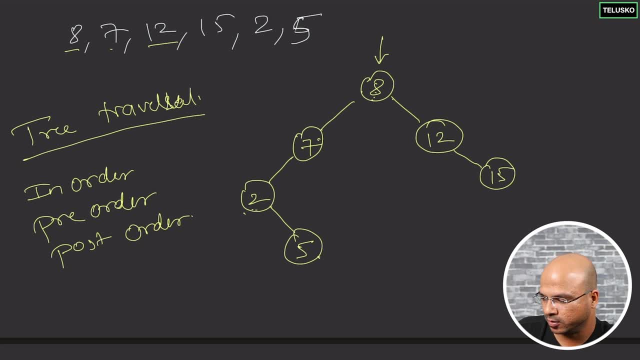 eight. but then we cannot work on the eight because that's an in order. then you go to the left one, because in order you first go for left hand side, left subtree, and then from seven. also you can't print 7 because 7 becomes a root node for the 2. so we have to go to 2 now. we don't have any left. 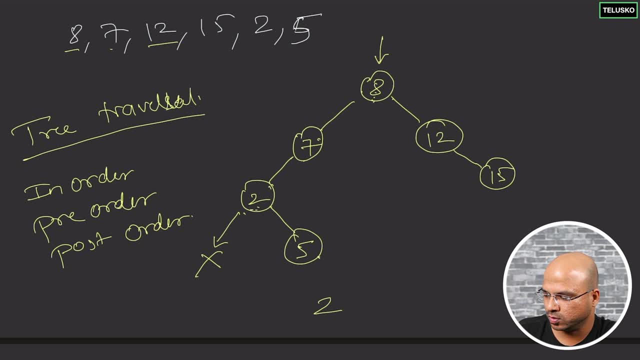 here. right, this is empty. so in this case you will first print 2. okay, so you will go for 2, but then you go for right. since we don't have a left, we print the root node, because we are considering this subtree now. so you will print 2 and then you will print 5. so here we have 5, then you go up. 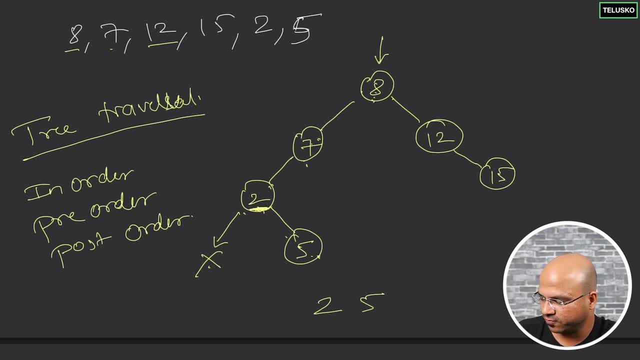 then you print 7 because we don't have anything. so that's apparent for 2, so we'll go for 7. then we print on the right hand side: we don't have anything right inside, right, so this is empty. then you go up, you print 8, then you go for the right hand side. right hand side is 12 on 12 left. 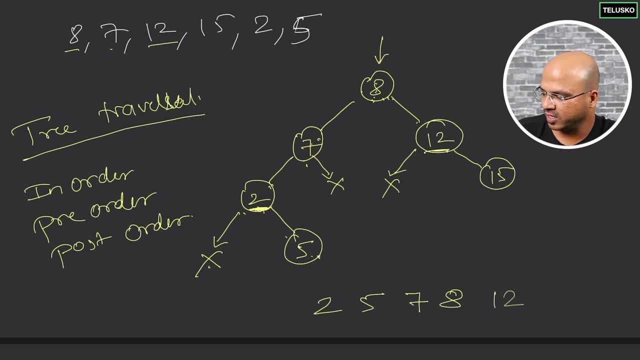 we don't have anything, so it will not print anything. but you can print 12 and then you can go for right hand side, which is 15, and if you observe, you got a sorted values. so that's why we use bst, which is sorted values. it is easier to search as well. okay, this is the in order traversal. 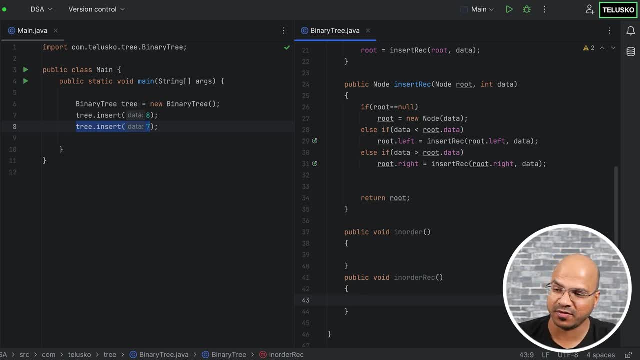 okay, so let's implement this. so how do we do it? so first, we'll start from the left hand side, but also we want to verify if the tree is empty. if the tree is empty, how will you print something, how will you travel and how do you know the tree is empty? by using the root element, so we can simply check if root, but how? 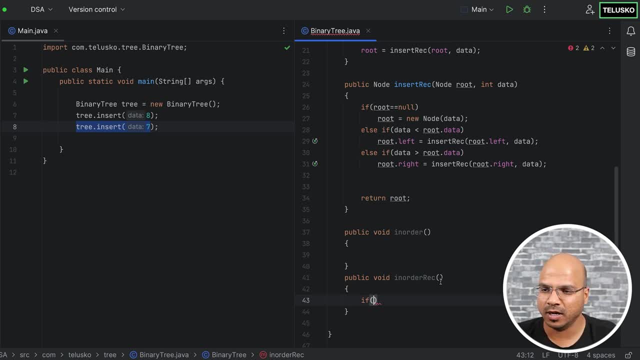 do you know the root? because root will keep changing depending on the tree, right? so we have to also accept root here. so we'll say node is root and then you check: if the root is not equal to null, then only you do it now. how will you do it now? first of all, this is a recursive function, right? 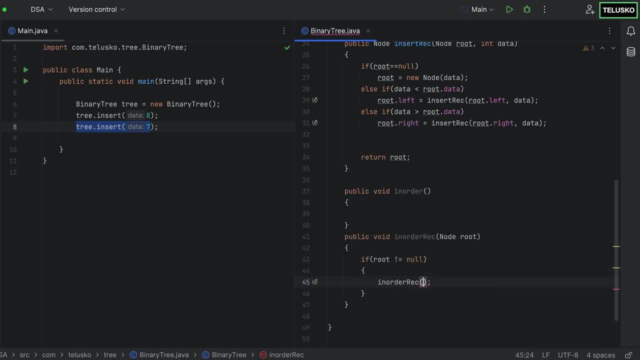 so basically you have to call itself. so we'll say in order, right, and then you have to start from the left hand side. so always start from left and then keep going till you find the last left element, okay, and then, once you do that, then you have to go for the middle one. middle one is root. 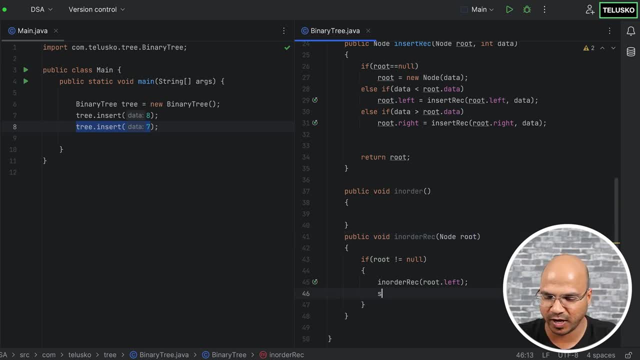 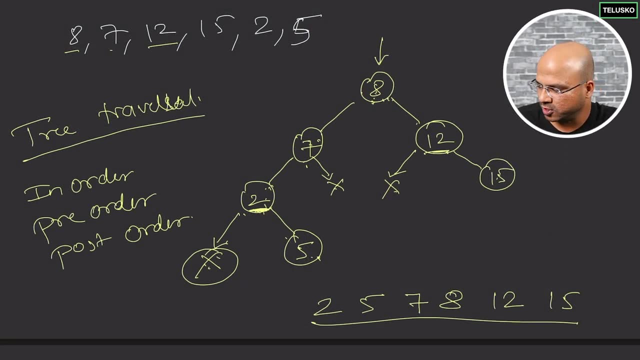 itself, which we got here right, so we can print this value here. so i will say print. and if you observe, for every node, for every sub tree, there is always a root node. if you observe, for eight, seven is left, right, but don't you think seven in this sub tree is a root node, so that's the. 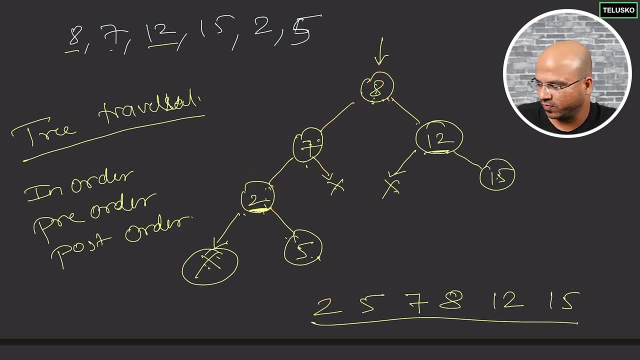 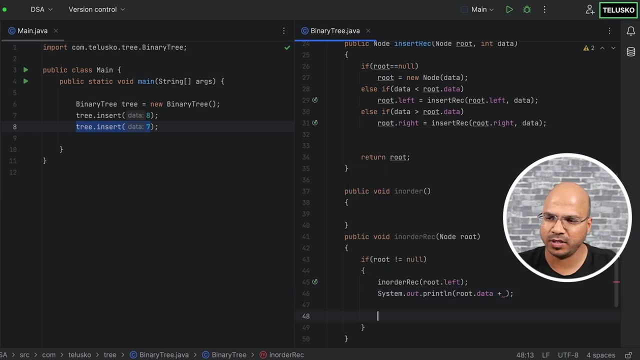 root we are printing. when you go to two, two becomes a root node. right, when you go five, five becomes a root node for their child, which we don't have- then we can. so we can print data here, so we can say root dot data and then we can print a space in between as well, just to differentiate.